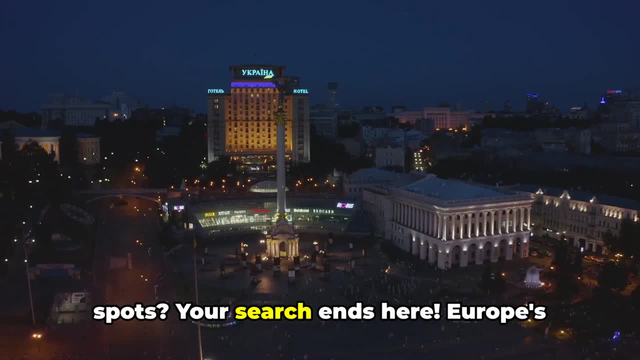 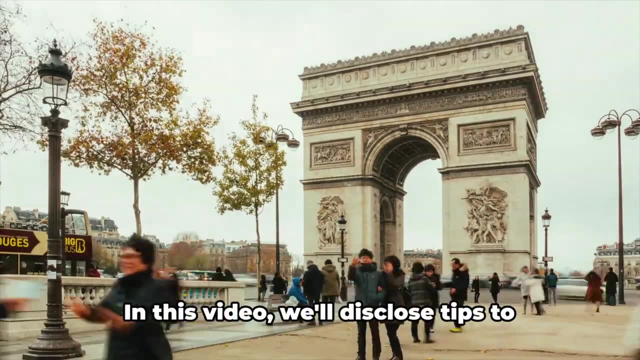 Searching for inexpensive European travel spots, Your search ends here. Europe's charm doesn't have to drain your wallet. Cities like Vienna and Sofia offer budget-friendly experiences. In this video, we'll disclose tips to economize your trip. Fasten your seatbelts as we dive into 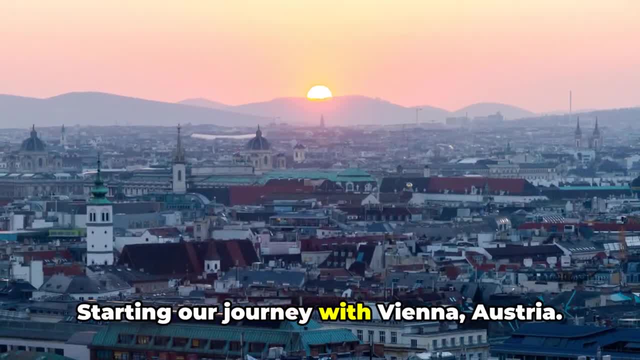 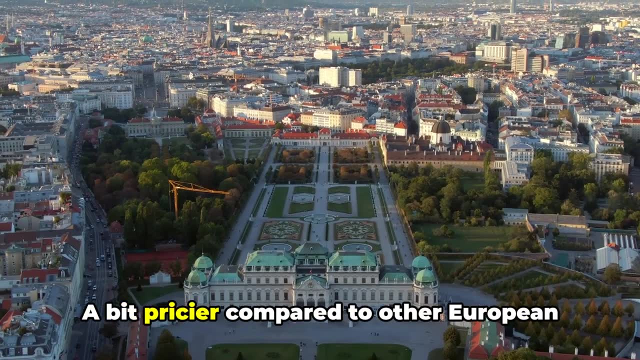 affordable European cities exploration, Starting our journey with Vienna, Austria, A city with grand palaces, first-rate museums. It's like stepping back in time, A bit pricier compared to other European cities, at an average of 80 euros daily, Yet its old-world charm makes it. 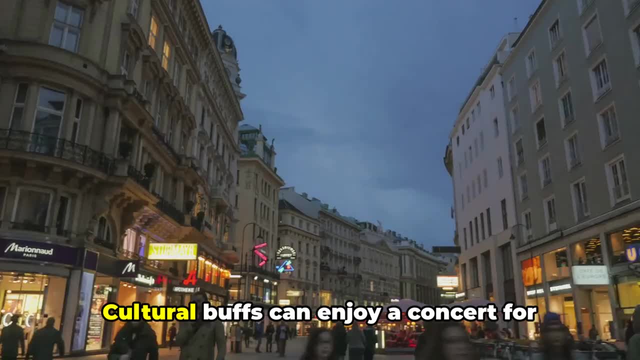 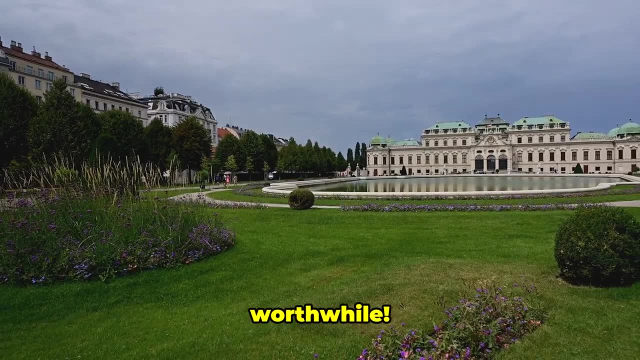 worth every penny. Traditional meals are pocket-friendly. Cultural buffs can enjoy a concert for 20 euros. Despite being costly on our list, Vienna's splendor makes every expenditure worthwhile. Next on our list, we find ourselves in the enchanting city of Prague, A vibrant mix. 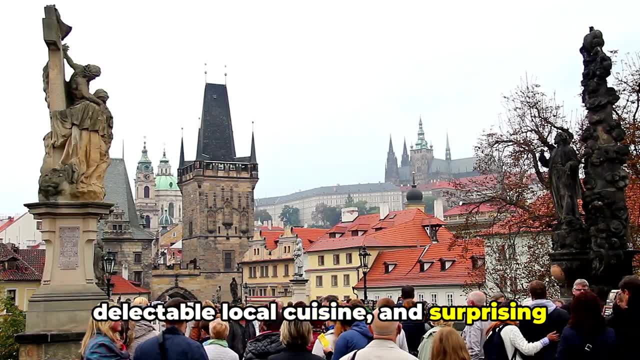 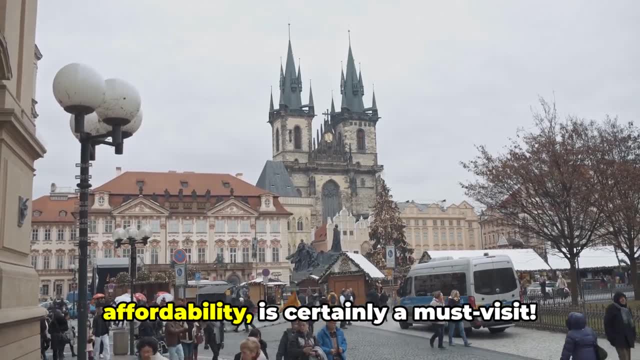 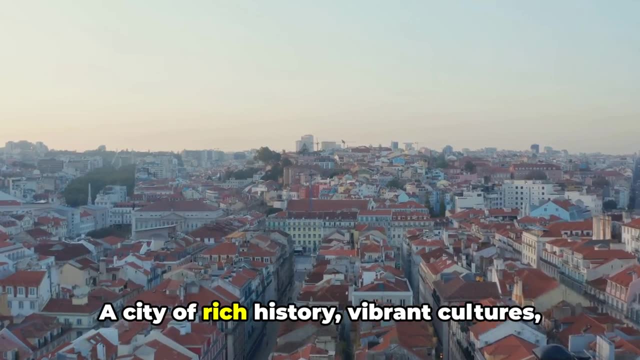 of ancient architecture, delectable local cuisine and surprising affordability make Prague a unique destination. Prague, with its captivating charm and affordability, is certainly a must-visit. Moving further down the list, we land in Lisbon, Portugal's vibrant capital, A city of rich history. 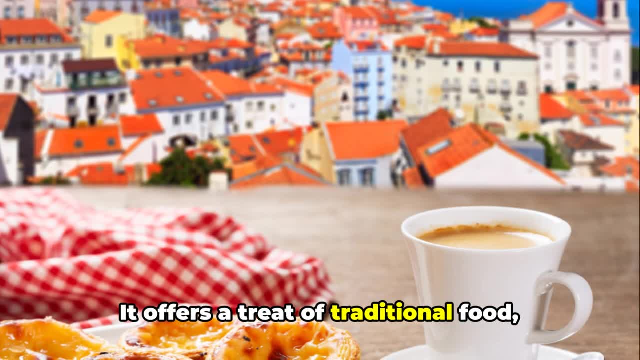 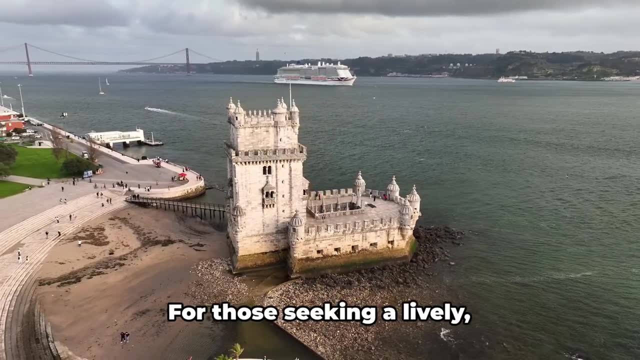 vibrant cultures and sensory delights. It offers a treat of traditional food, street art and affordable attractions like Tram 28 and Bellum Tower. Accommodation is plentiful and cost-effective. For those seeking a lively, budget-friendly destination, Lisbon is your. 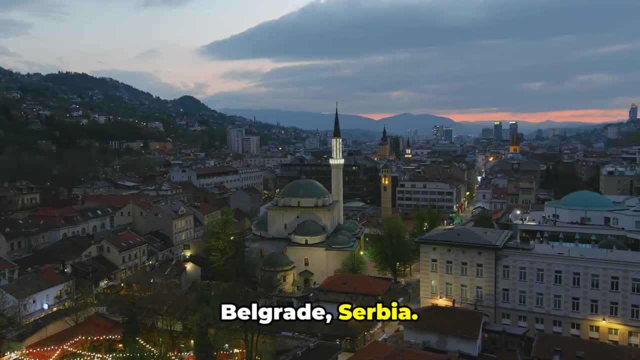 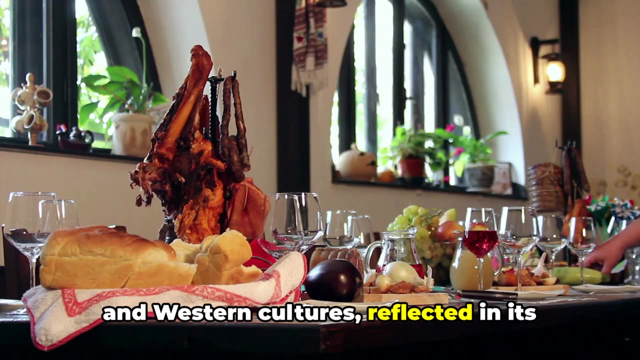 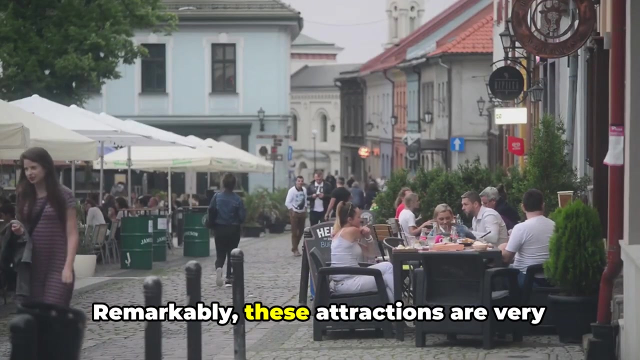 answer. Next, we venture off the beaten path to Belgrade, Serbia, This undiscovered gem. the country's capital is a fascinating blend of Eastern and Western cultures, reflected in its architecture and gastronomy. Its affordable local food and pulsating nightlife are well-known. Remarkably, these attractions are very affordable, making 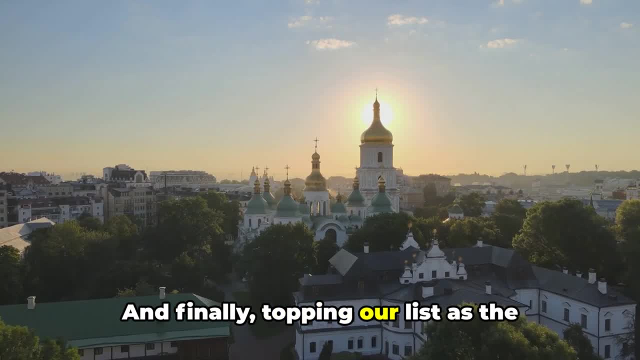 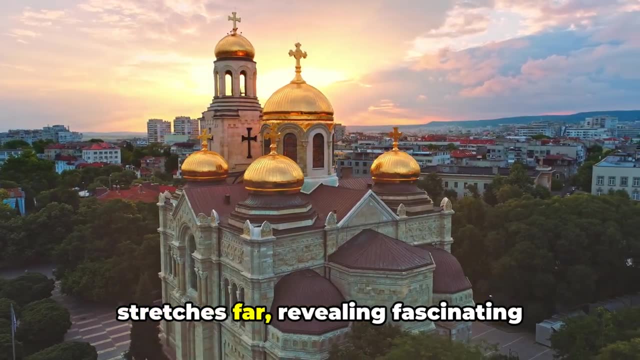 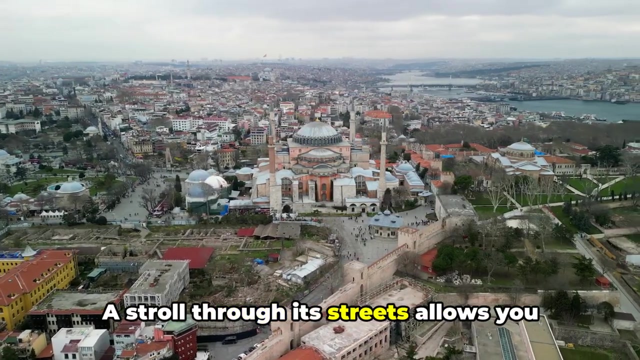 Belgrade, ideal for budget travelers And finally, topping our list as the cheapest European city to visit. we have Sofia, Bulgaria. This city is a gem where your dollar stretches far, revealing fascinating sights and a rich history. It's a city that takes pride in its past. A stroll through its streets allows you to 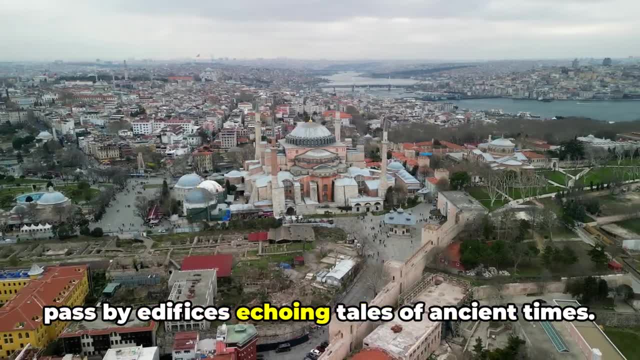 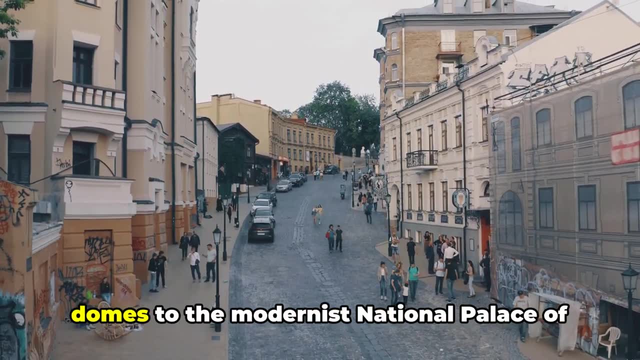 tread on centuries-old cobblestones and pass by edifices echoing tales of ancient times. Sofia's architecture is a feast for the eyes, From Alexander Nevsky Cathedral's golden domes to the modernist National Palace of Culture. it's a visual gallery The city even offers.